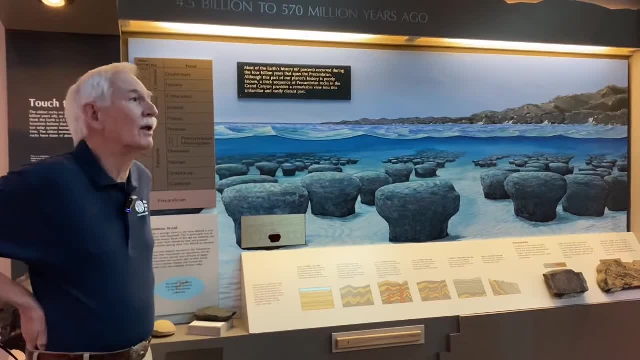 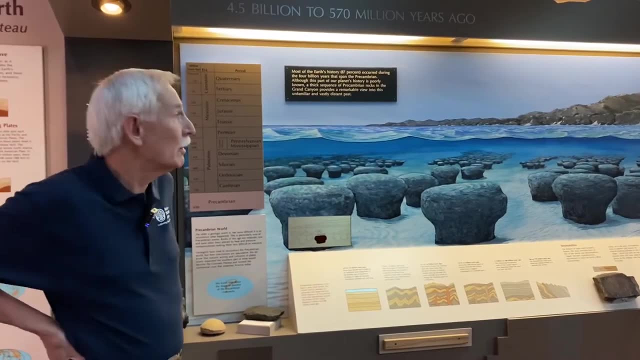 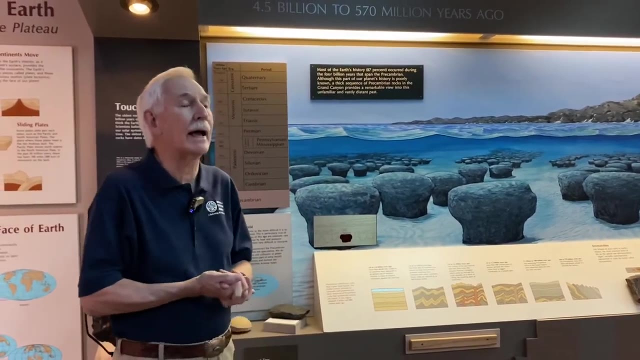 Because we usually think of things in terms of life, But this is before life. This is before life really existed here on planet Earth or on the Colorado Plateau of the future. We did, however, have a consolidation of all those rocks that were laid down or created with the formation of the Earth. 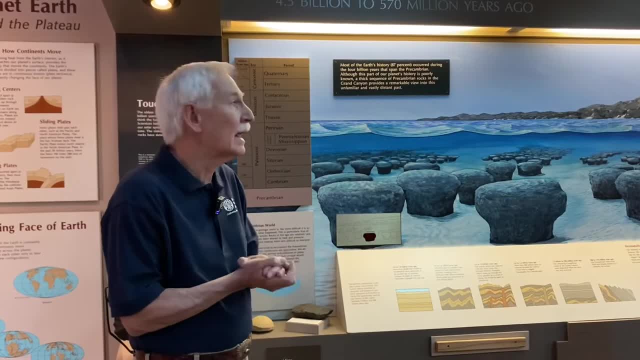 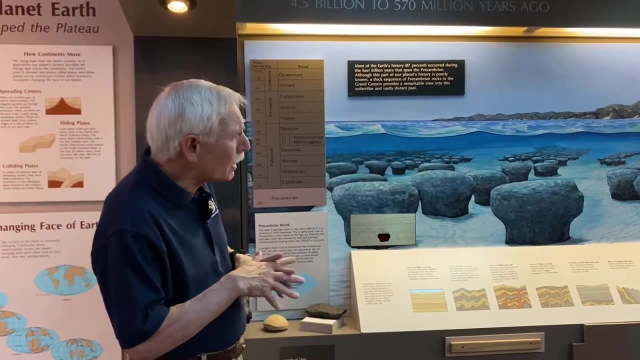 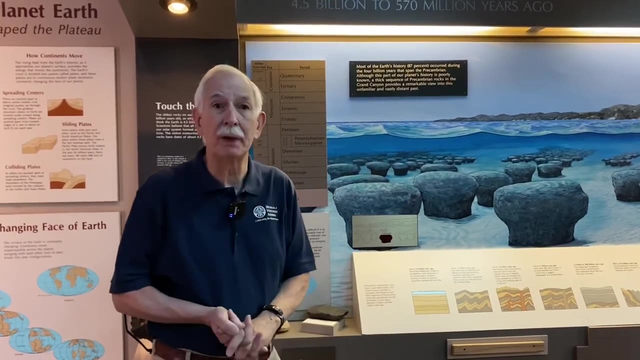 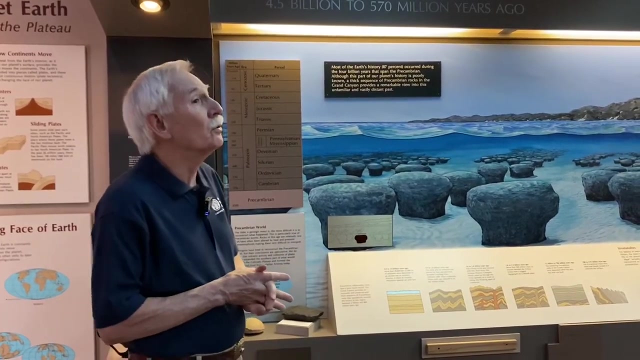 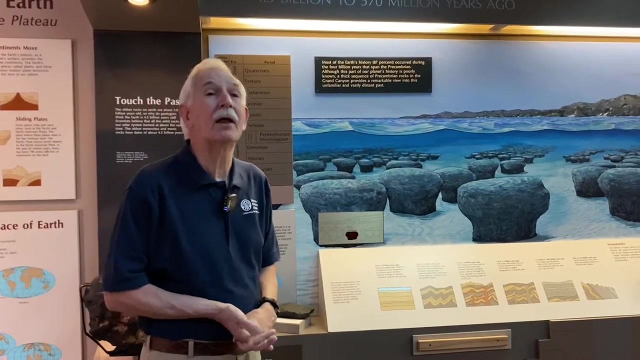 The heat that they generated has now dissipated And we're beginning to see a more normal world. like we might expect to see, The rock layers have begun to form into the continental plates that we're all familiar with. The plate that we're located on, the North American plate, actually was joined together with the plates that will become Australia, Antarctica and China. 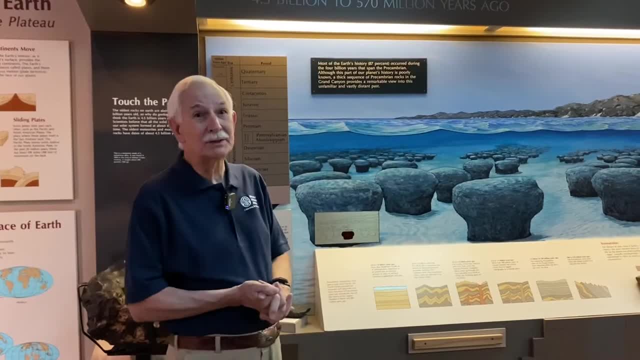 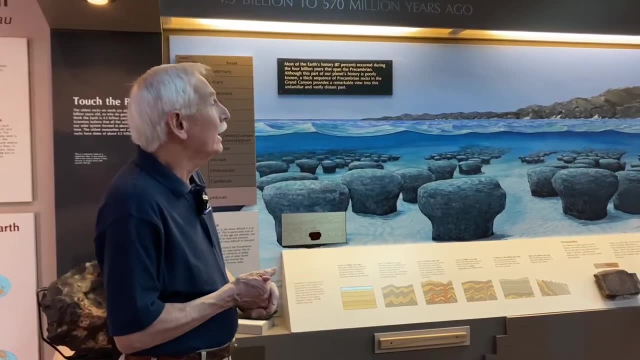 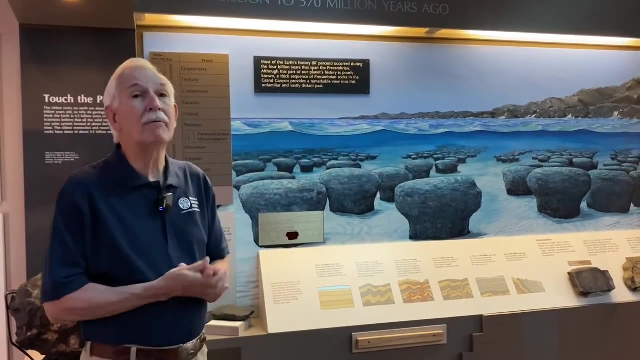 Imagine that We were once attached to Australia, Or Australia was attached to us back in those days. All of these plates came together Into a supercontinent called Rodinia that existed during the latter days of the Precambrian. So we have rock surfaces, land surfaces. 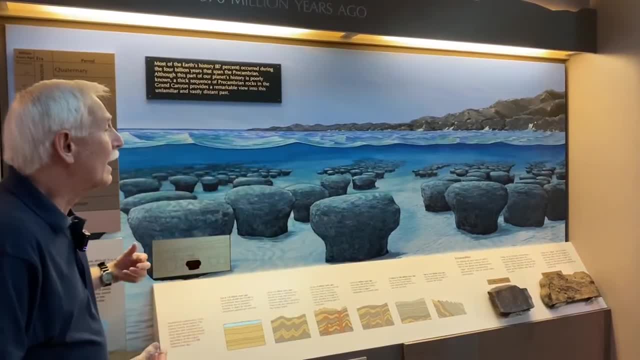 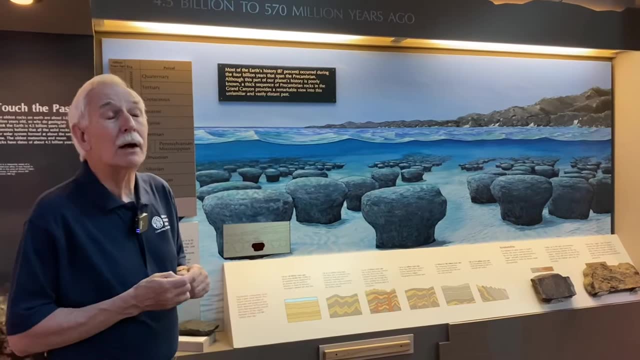 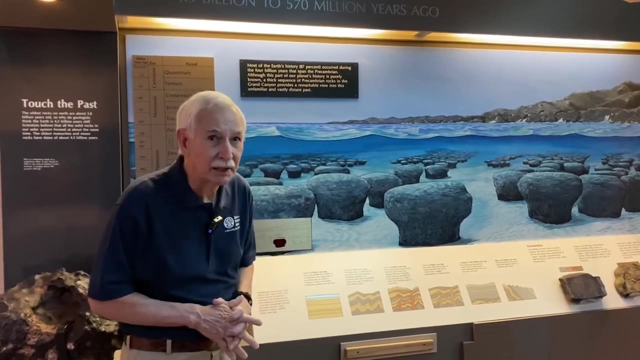 We have the oceans formed, But what we don't have is life, except for single cell organisms. The life that we are accustomed to has to do with plants and animals- Plants and animals that consume oxygen. Unfortunately, in most of the Precambrian, there was no oxygen in the air. 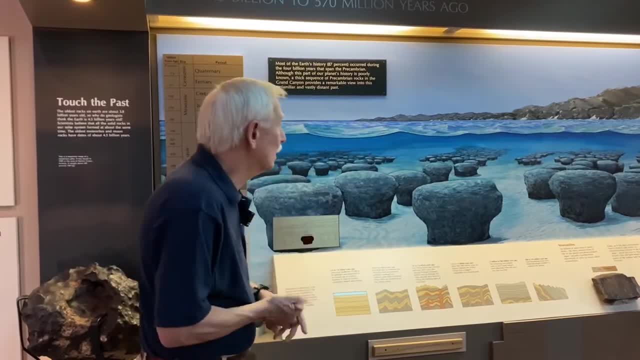 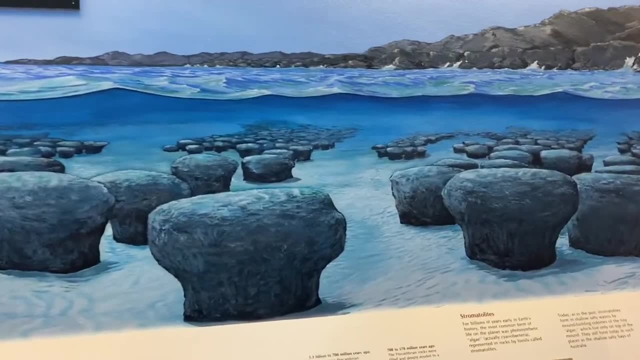 Carbon dioxide for the most part. So take a look at these little toadstool-like items you see here in the water. They're called stromatolites And it's due to the stromatolites that the oxygen that would make life as we know it possible. 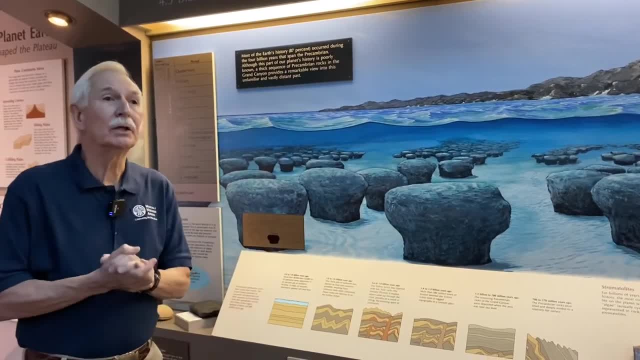 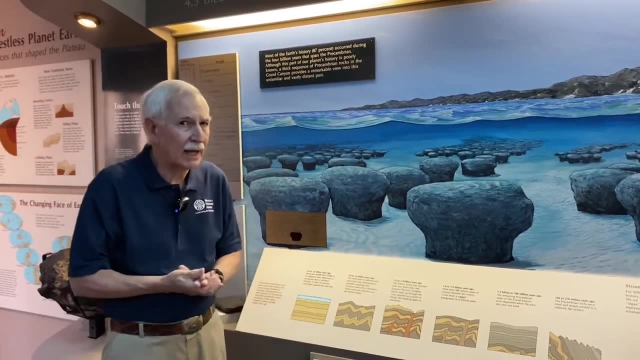 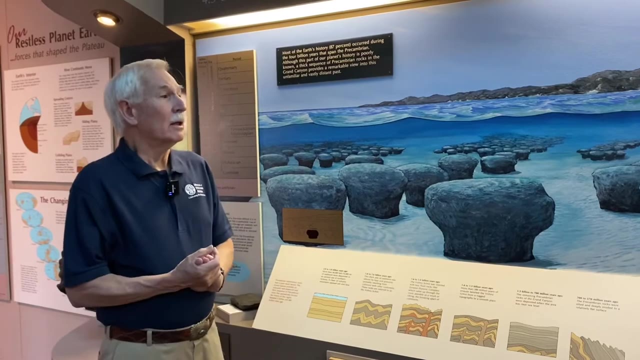 we can attribute it to a plant. The function of these stromatolites? And what are they? They are mats layers of blue-green algae, a cyanobacteria, that consume, eat carbon dioxide. The carbon part of the carbon dioxide is their food.